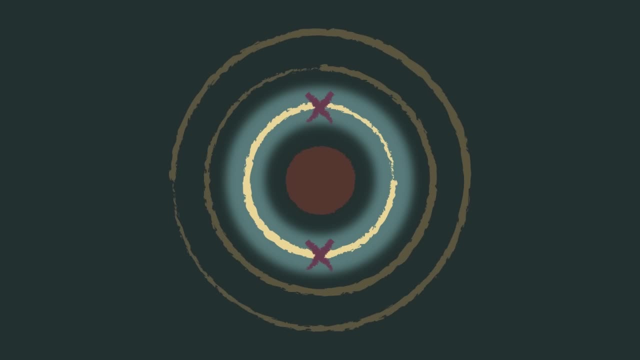 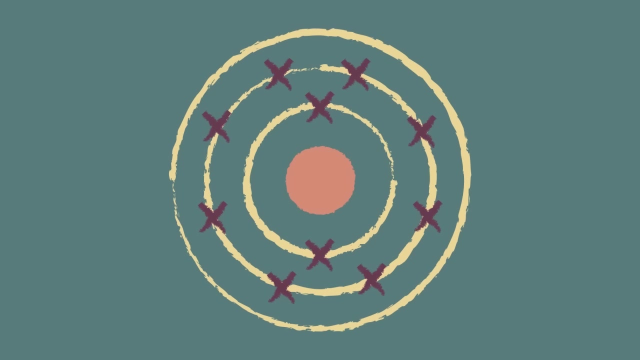 lowest available shell, And whenever a shell is full, the next electron to be added goes into the next shell, And that's pretty much it. All you need to know is how many electrons can occupy each shell and at this level you only need to know. 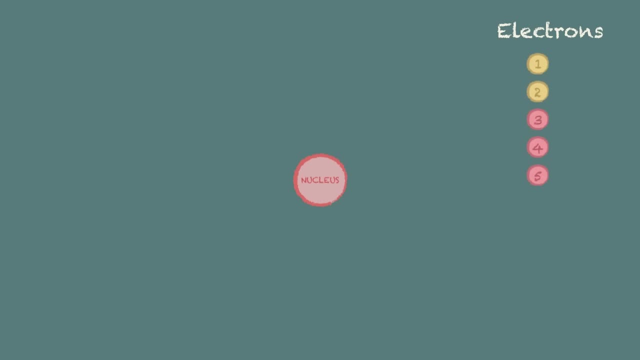 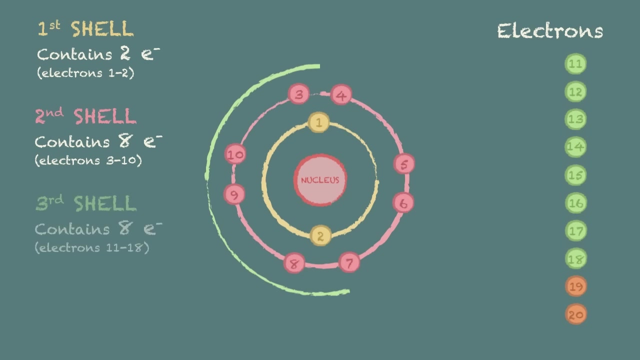 the rules for the first 20 elements. The maximum numbers are as follows: The first shell can contain a maximum of 2 electrons, The second shell up to 8 electrons, The third shell also has a maximum of 8 electrons, And the 19th and 20th electrons. 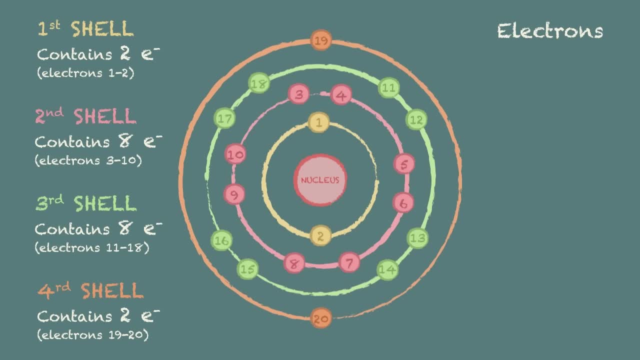 go into the 4th shell And this would actually represent a calcium atom. Note that as we fill up each level, we've been drawing the electrons evenly spaced out on each shell. This is to keep the diagrams tidy and make it easier to count the electrons. 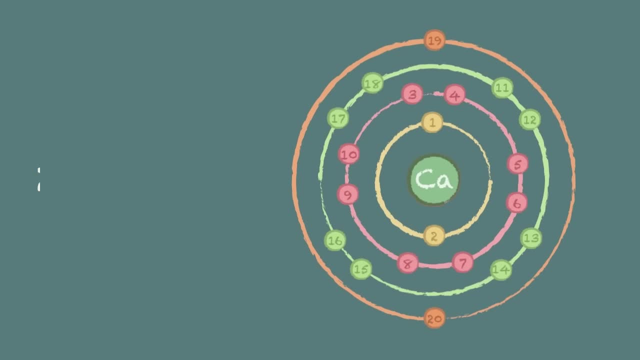 And, what's more, there's a shorthand way of writing this down: 2,, 8,, 8,, 2.. The first number represents the inner shell, or lowest energy level. The full stop shows how the electrons are separated between the shells. 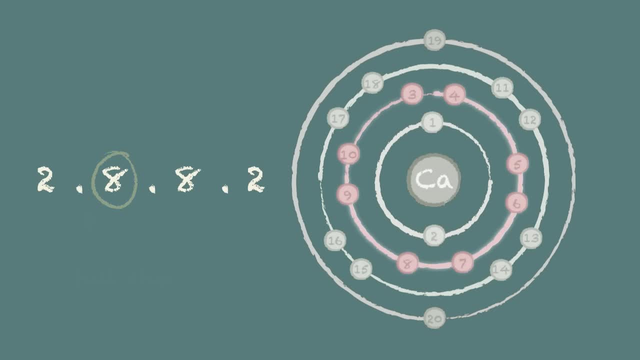 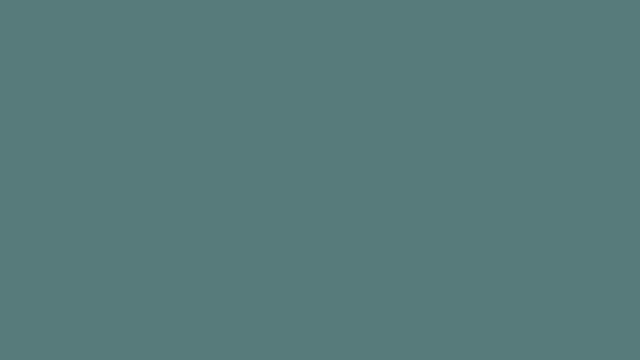 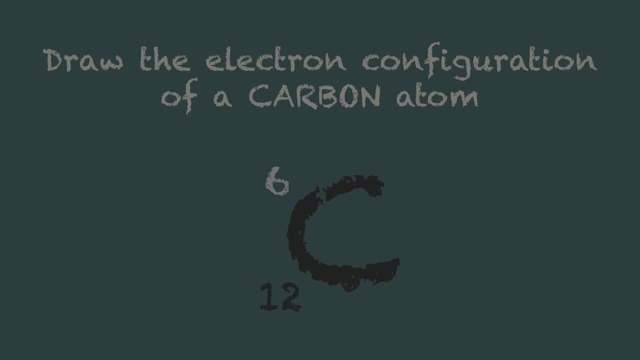 The second number tells us how many electrons are in the next shell, followed by the third and fourth shells. And so now it's your turn. I'd like you to draw the electron configuration of a carbon atom. Pause the video, find a piece of paper and have a go. 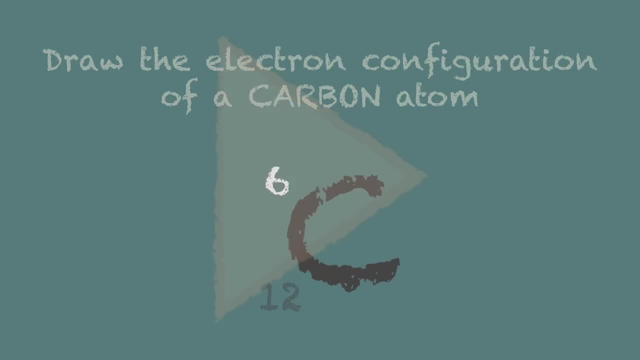 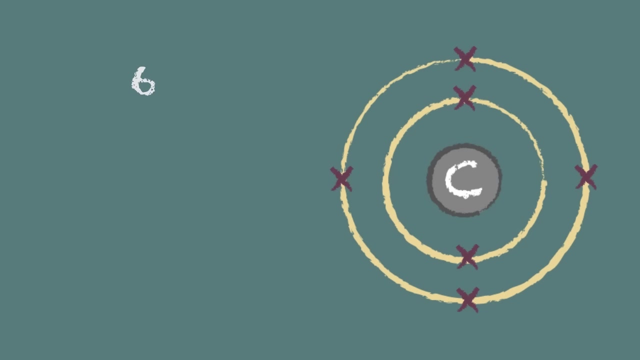 And here is what it should look like: 1,, 2,, 3,, 4.. And here is what it should look like. It has a full first shell and four electrons in the outer shell. Did you get it right? 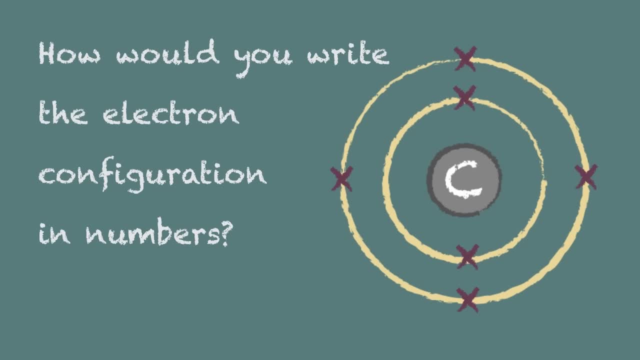 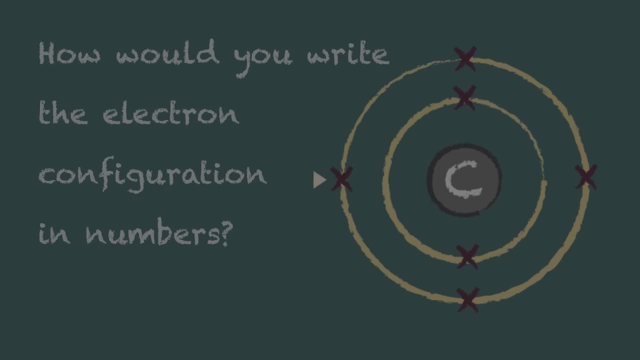 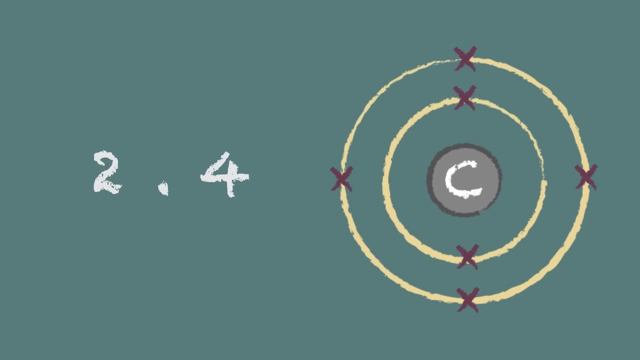 Now, how would you write the electron configuration in numbers for this atom? Pause the video again or rewind if you need to have a think about this. The answer is that it would be written 2, dot 4.. And now that you have covered the, 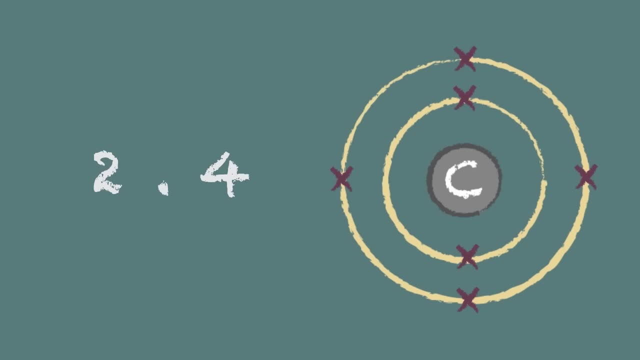 basics of drawing electron configuration, let's move on to the next step, 2, dot 4.. And now that you have covered the basics of drawing electron configuration, you'll be ready to tackle our lesson: Electron Configuration of the First 20 Elements. 1,, 2,, 3,, 4..